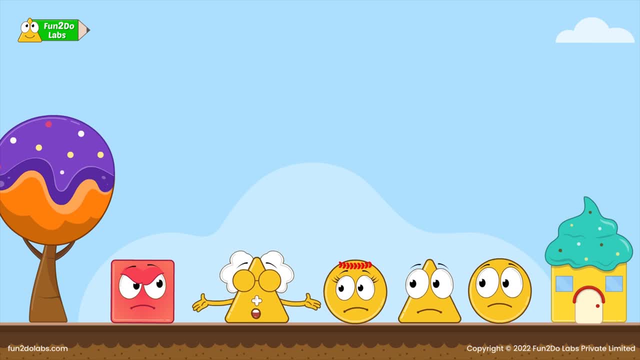 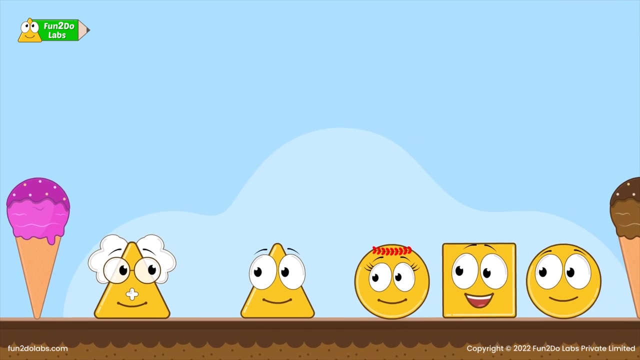 Uncle Matt then asks Squirrel to take a deep breath and count from 1 to 10 backwards. Voila, Squirrel is calm and normal now. Uncle Matt helps the kids in deciding who ate more ice creams. Treeho, how many ice creams did you eat? 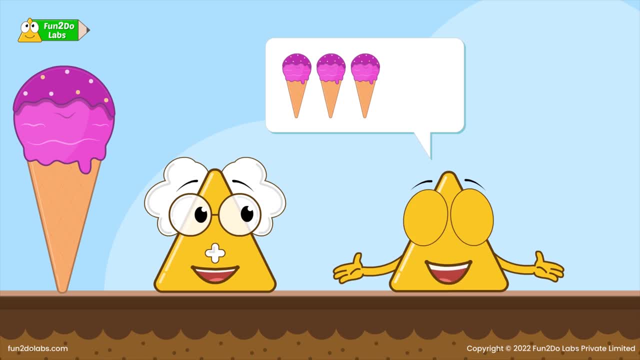 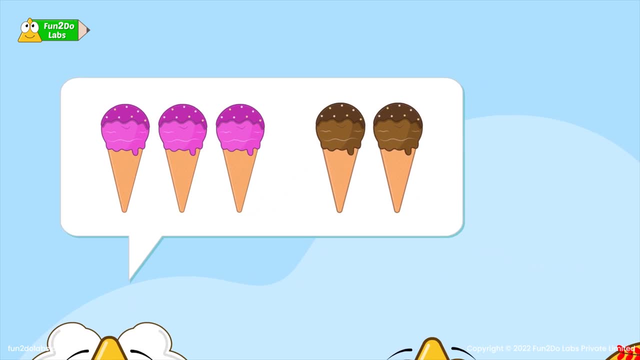 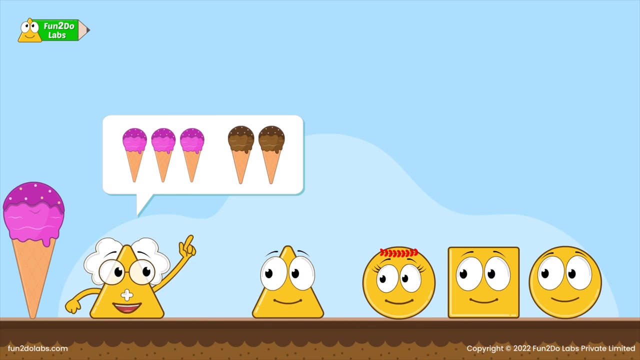 Umm, I ate three pink ice creams first and two brown ice creams later. But how many did I eat all together, Taking some pink and brown ice creams? Uncle Matt explains: So you ate these three first and these two later. Now can you tell me how many you ate all together? 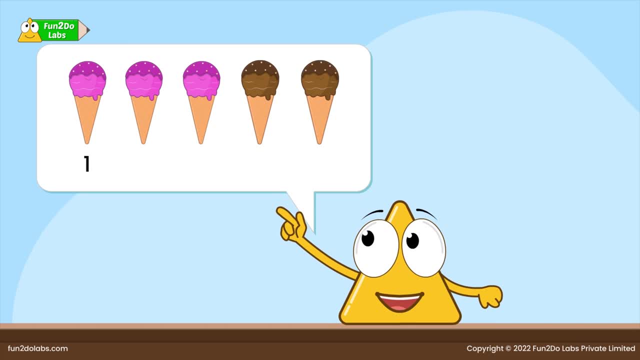 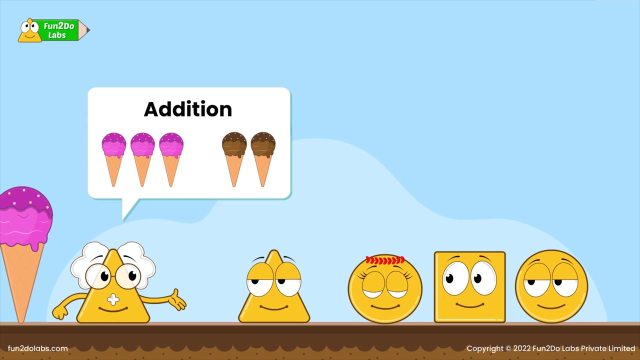 Treeho counts excitedly: One, two, three, four, five. I ate five ice creams all together. Well done, Then. how many did you eat? This method of putting two or more things together is called addition. We show addition using the plus symbol. 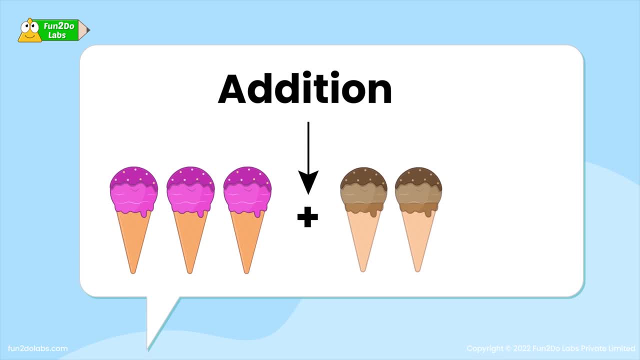 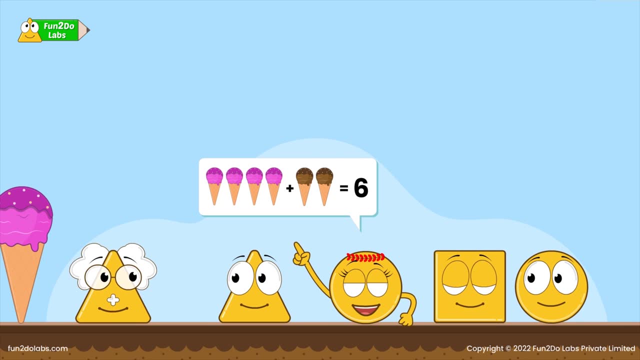 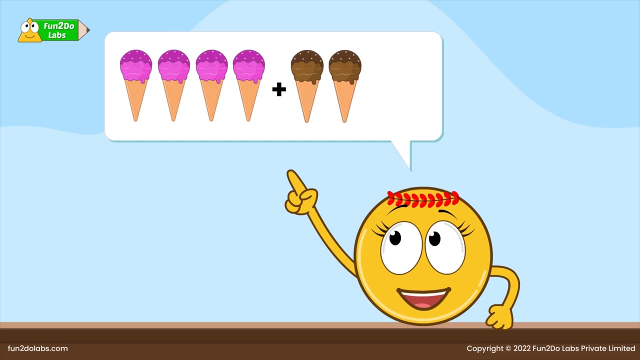 So we say: three ice creams plus two ice creams is equal to five ice creams. Sira is intrigued and wants to try addition herself. She says: I ate four pink ice creams and two brown ice creams. She quickly grabs some ice creams and starts adding. 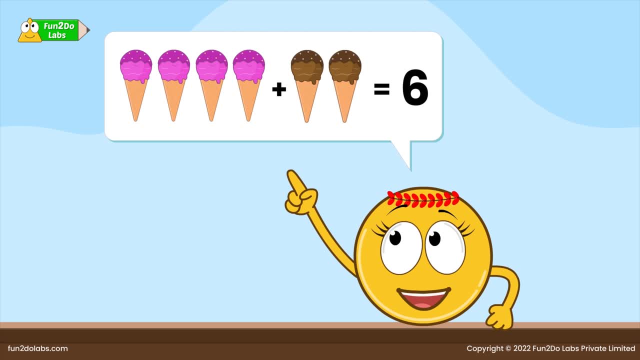 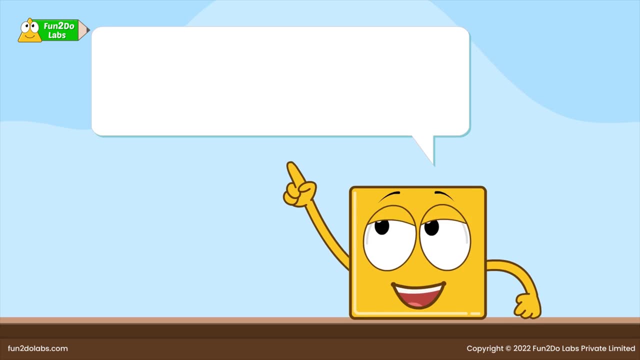 Sirha ate six ice creams all together. Following Sirha, Sirho and Squarro also decide to find out for themselves. Squarro ate three pink ice creams and four brown ice creams, So he ate seven ice creams all together. Sirho ate two pink ice creams and two brown ice creams. 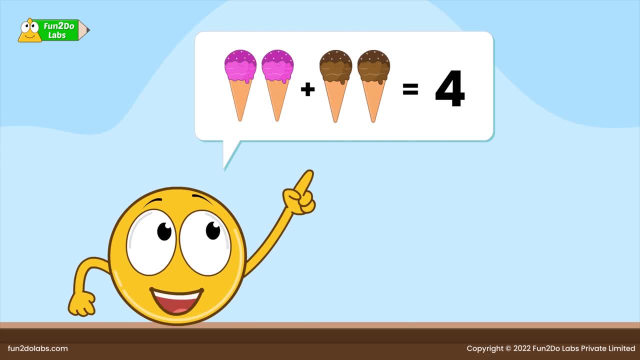 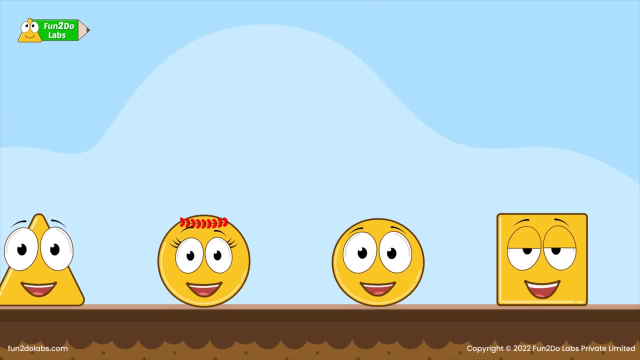 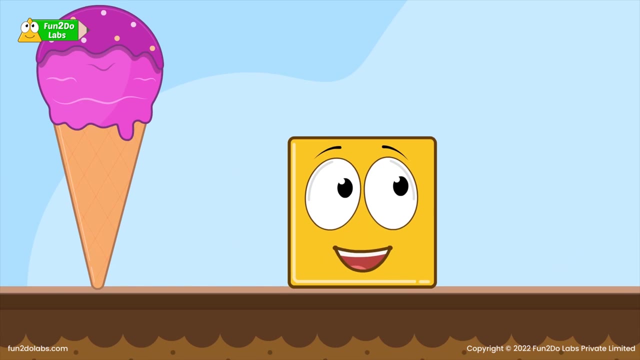 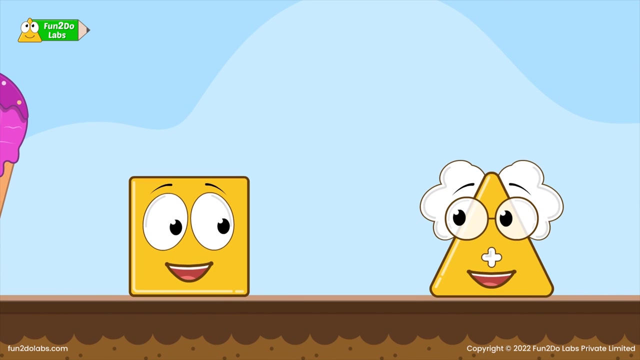 So he ate four ice creams all together. Treeho ate five, Sirha ate six, Sirho ate four And Squarro ate seven ice creams. Clearly, Squarro is the winner. Squarro is elated. He apologizes for his bad behavior and thanks Uncle Math for teaching him a simple anger management trick.